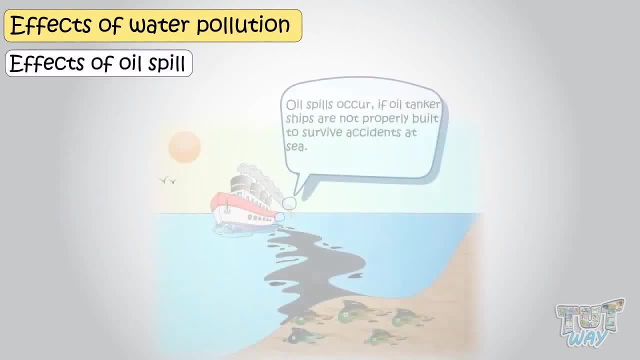 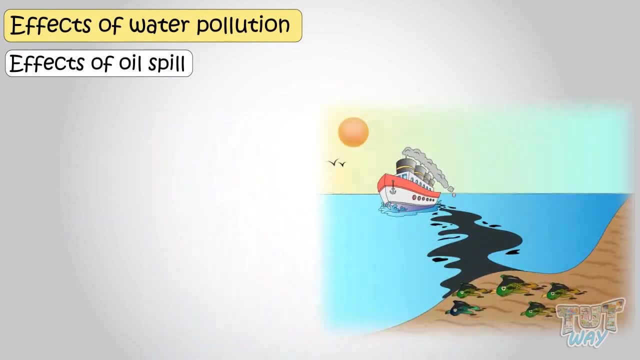 Oil spills occur if oil tanker ships are not properly built to survive as a result of polluted water. This causes accidents at sea. The oil spills devastate ecosystem and also effects tourism. Oil spills affect the coastal community rather than the people responsible for the oil spill. 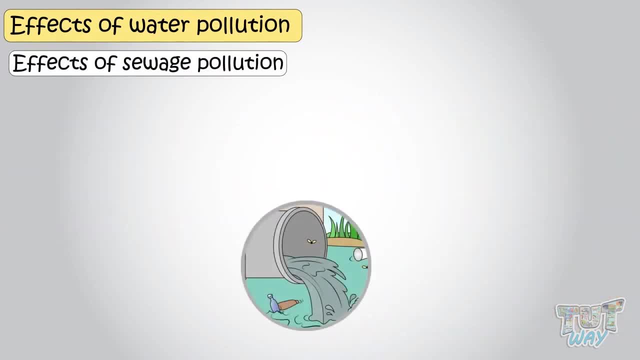 Disposal of sewage waste in water bodies affects us all, as it pollutes the water in water bodies and people who bathe or surf in such waters may fall victim to this. The water is contaminated by algae. Such waters may fall ill. 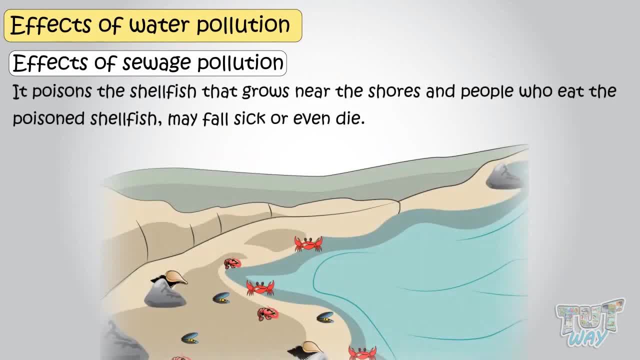 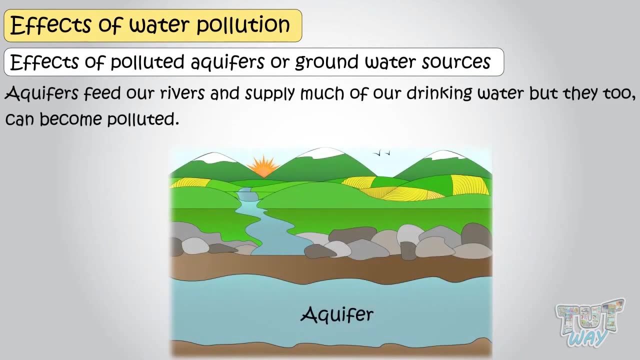 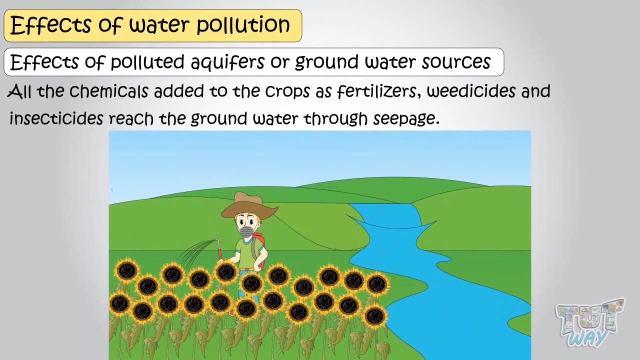 It poisons the shellfish that grows near the shores, and people who eat the poisoned shellfish may fall sick or even die. Aquifers feed our rivers and supply much of our drinking water. They too can become polluted, as all the chemicals added to the crops as fertilizers, weedicides, insecticides. 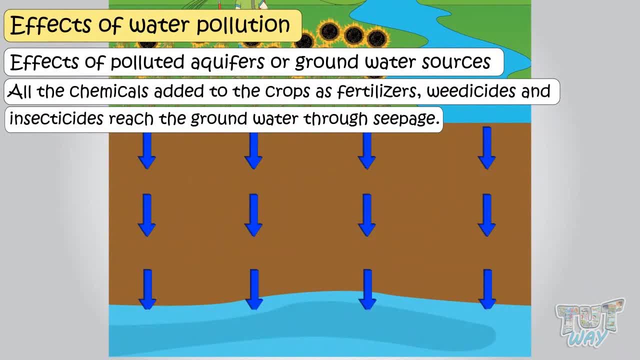 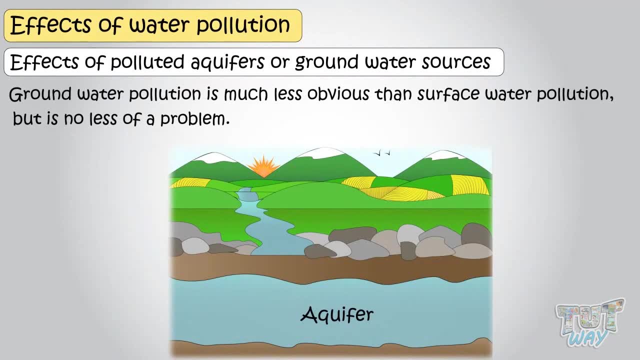 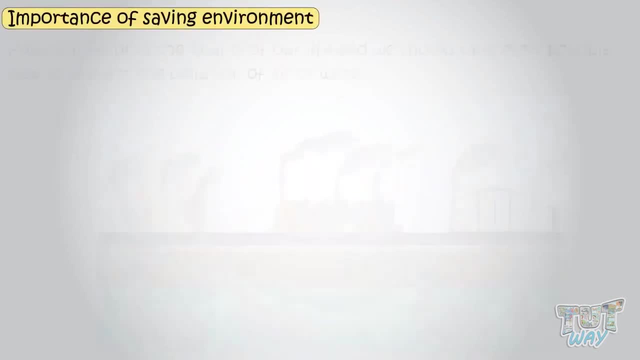 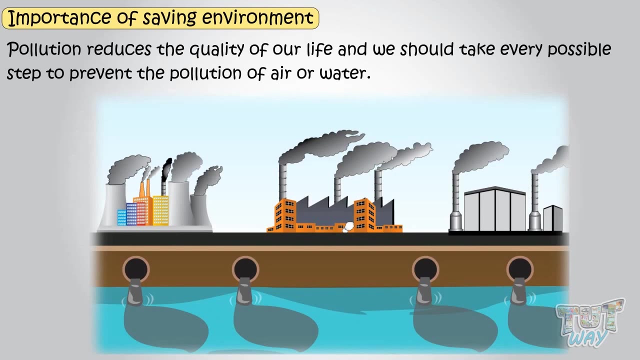 reach the groundwater through seepage. Groundwater pollution is much less obvious than surface water pollution, but is no less of a problem. So, kids, polluting environment reduces the quality of our life and we should take every step to prevent the pollution of air or water. 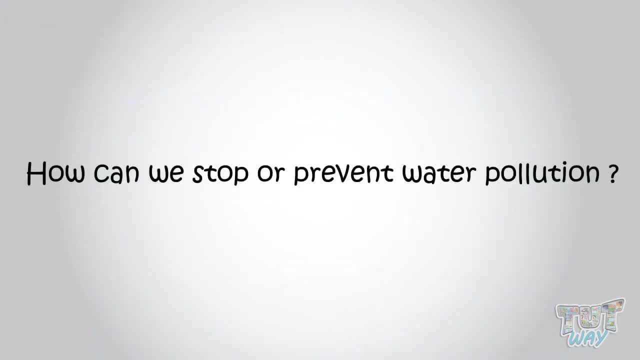 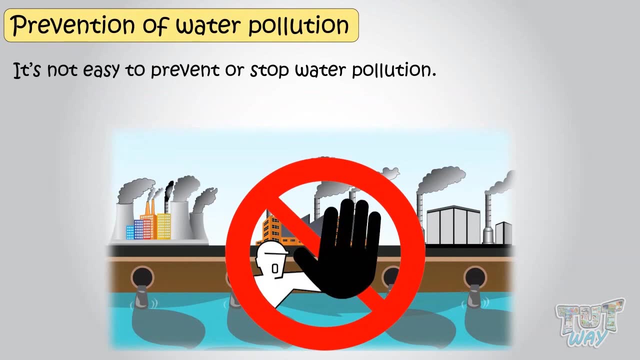 Now let's see how we can stop or prevent water pollution. It's not easy to prevent or stop water pollution. We need to take several steps in different spheres. Let's learn a few steps that can be taken to prevent water pollution, Making people aware of the problem. 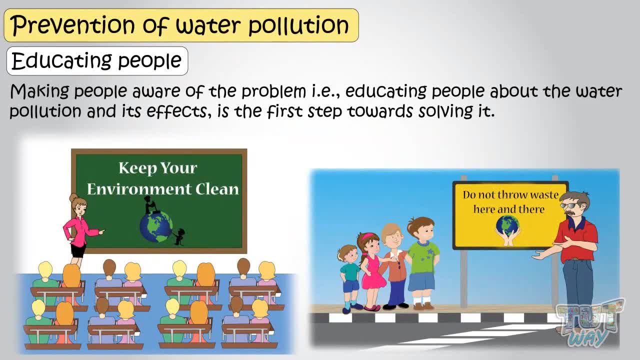 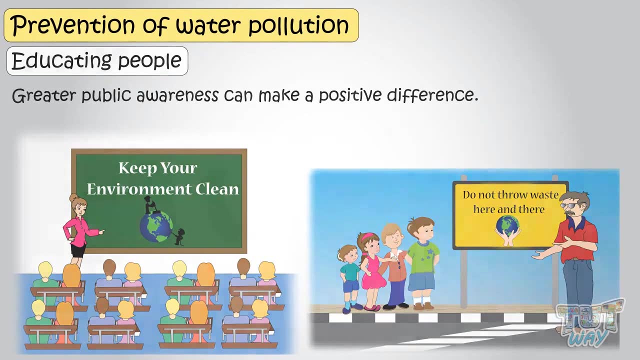 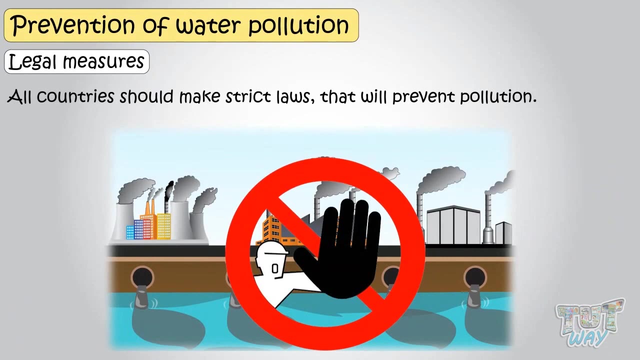 that is, educating people about the water pollution and its effects is the first step towards solving it, As greater public awareness can make a positive difference, Making laws to prevent water pollution. All countries should make strict laws that will prevent pollution, For example, 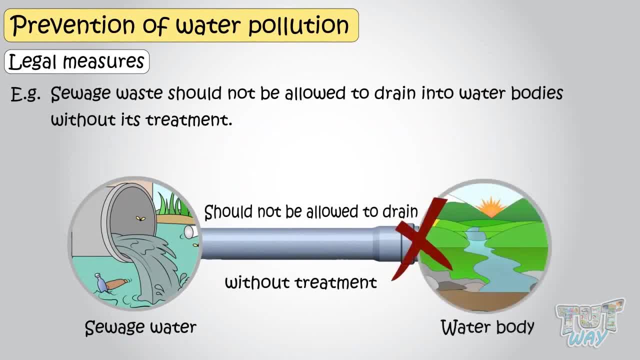 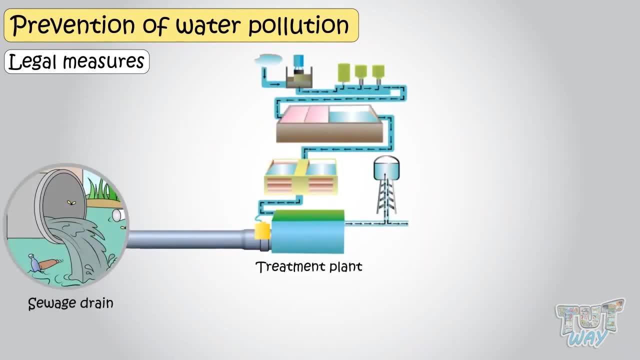 sewageways should not be allowed to drain into water bodies without their treatment. All the sewage drains should first lead to treatment plants. sewage water is treated to make it free from contaminants, and then only it should be discharged into any water body. Water pollution has transboundary nature. 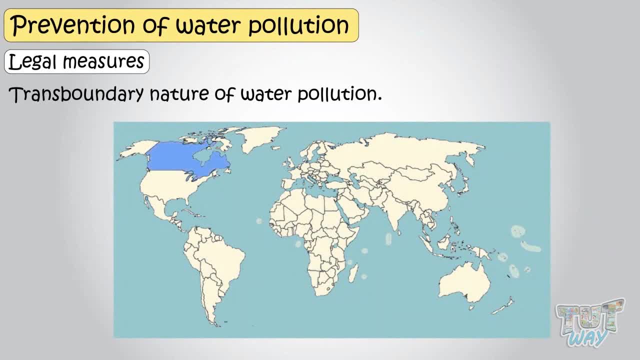 that is, waste discharged by one country may affect the other countries also, As big water bodies like seas and oceans are common, they don't belong to any particular country, So laws are required to be made on international or continent level. Now let's learn some economic measures to prevent and reduce water pollution. 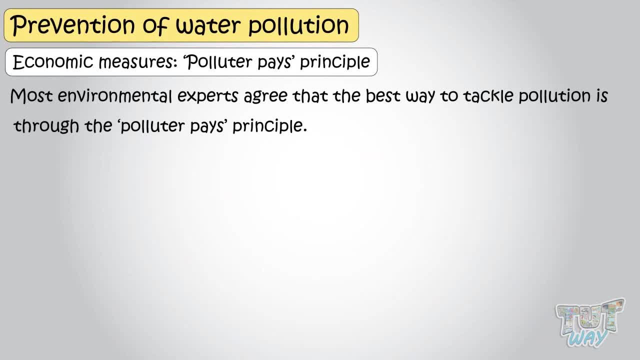 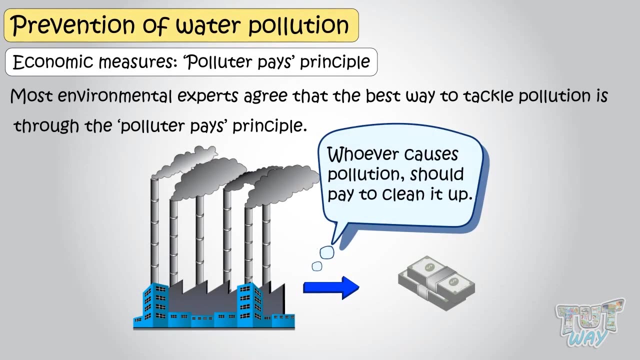 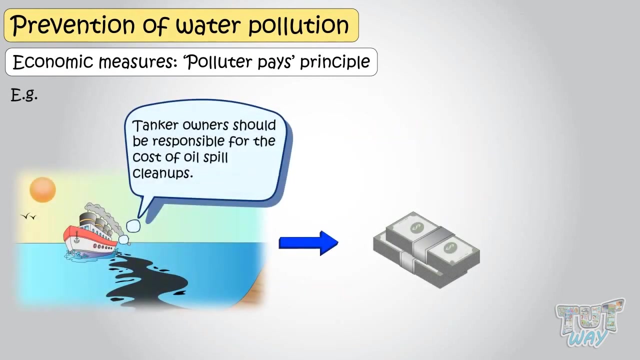 Most environmental experts agree that the best way to tackle pollution is through something called the Polluter Pays Principle. This means that whoever causes pollution should have to pay to clean it up one way or another. Tanker owners should be responsible for the cost of oil spill cleanups. 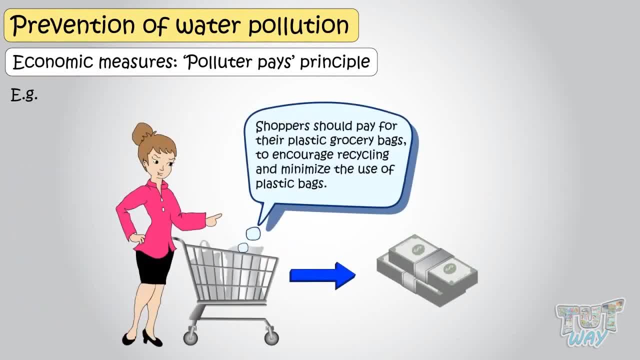 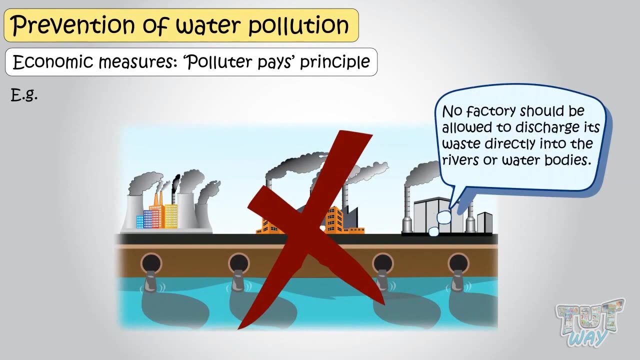 Shoppers should have to pay for the plastic grocery bags. to encourage recycling and minimize the use of plastic bags. No factory should be allowed to discharge its waste directly into the water Or any water body without treating the waste water, That is, without removing the harmful substances from it. 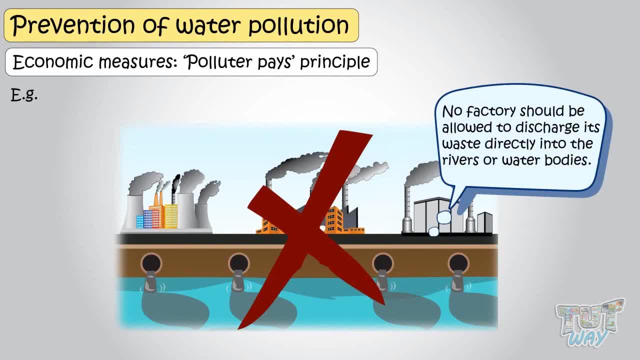 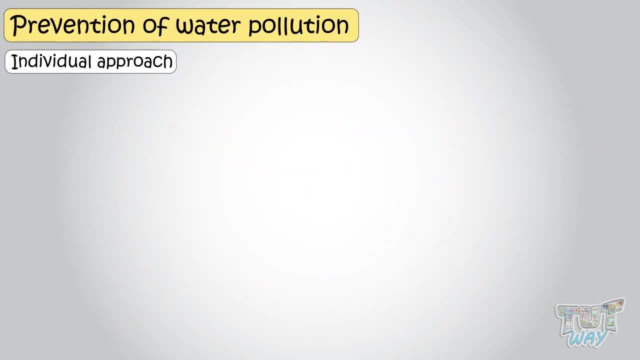 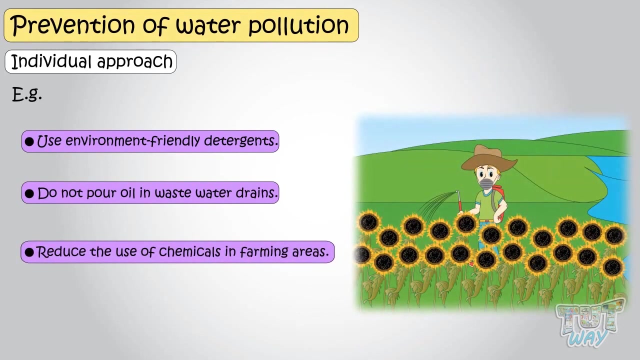 Now let's learn what can be the individual approach to reduce pollution. That is, what steps can we take to reduce water pollution? We should use environment friendly detergents. We should not pour oil in waste water drains. We should reduce the use of pesticides. 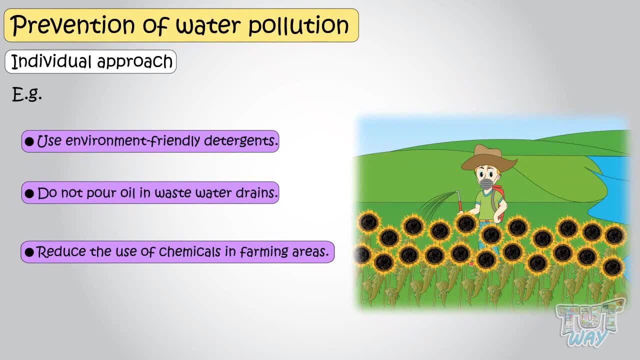 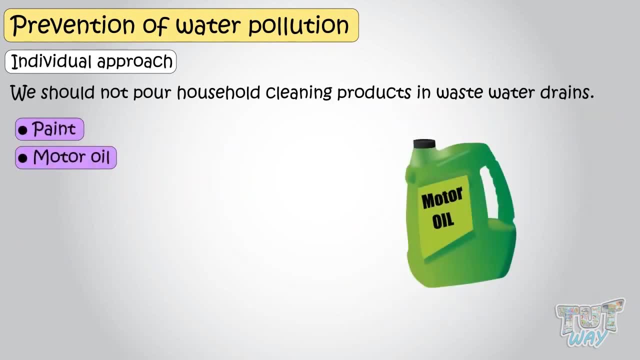 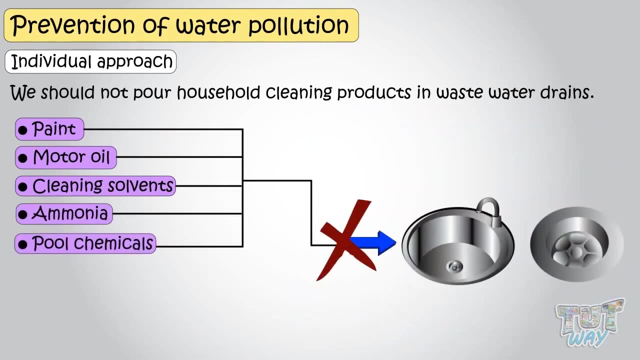 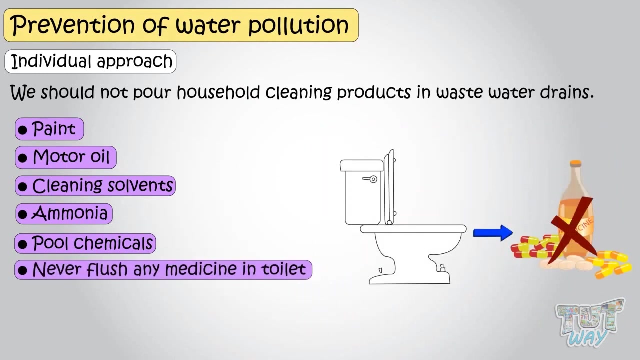 weedicides and fertilizers in farming areas. We should not pour household cleaning products like paint, motor oil, cleaning solvents, ammonia, pool chemicals in the drains. as we know, drains too ultimately leads to the water bodies. Never flush any medicines in toilets.